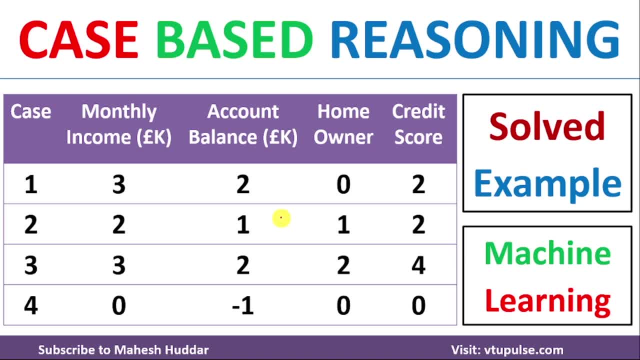 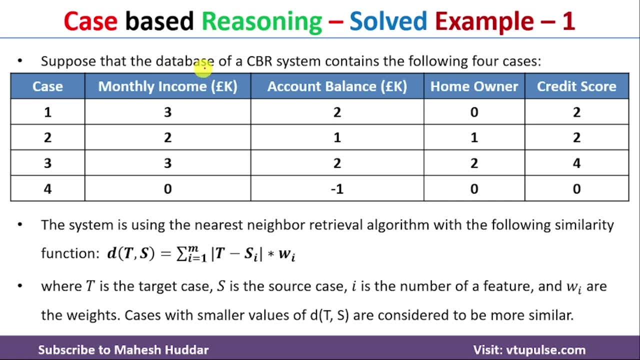 of a target variable for the given example. This is the solved example number one. The link for other examples is given in the description below. In this case, we have been given a database of a CBR system containing four cases, Each of these particular four cases containing: 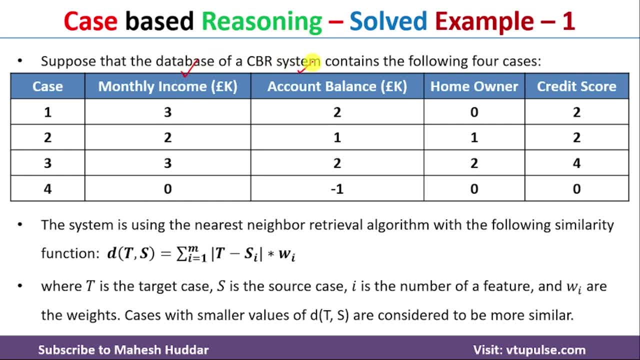 three attributes. The first one is monthly income. Second one is account balance. Third one is homeowner. In this case, the credit score is the target variable. Given this particular data set, we need to use the nearest neighbor retrieval algorithm to find the similar example. 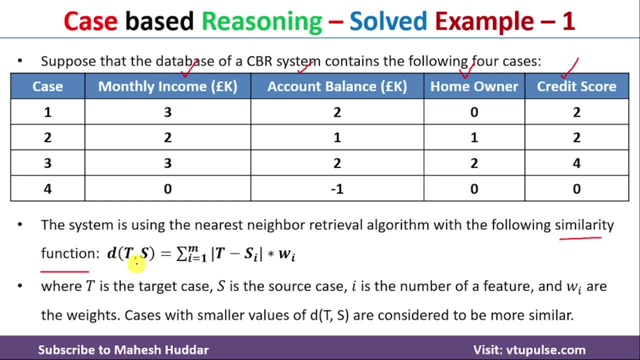 In this case, similarity function is also given. The first case given to us, ie d of t, s is equal to summation of i is equal to 1 till m, where m is the number of cases. Cardinality of t minus si multiplied by wi. Here t is: 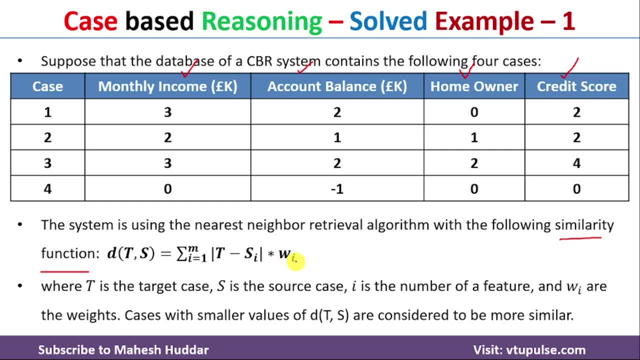 the target case. si is the source case, wi is the weight assigned to each of these particular variables. The cases with the smaller value of this distance, ie, d of t, s, are considered as more similar cases here. This is the target case given to us. The second case given to: 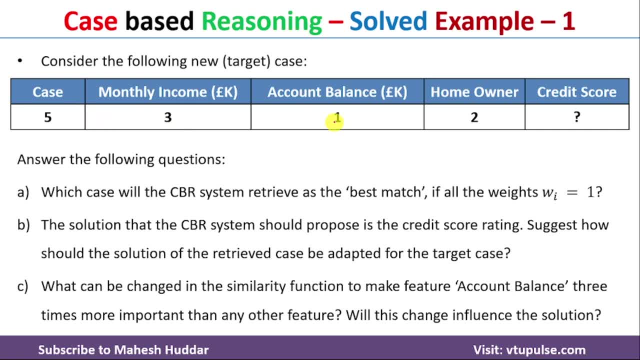 us. In this case, monthly income is equal to 3, account balance is equal to 1,. homeowner is equal to 2.. Given this particular target case, we need to find the credit score for this particular target case. Given this particular information, we need to answer the following. 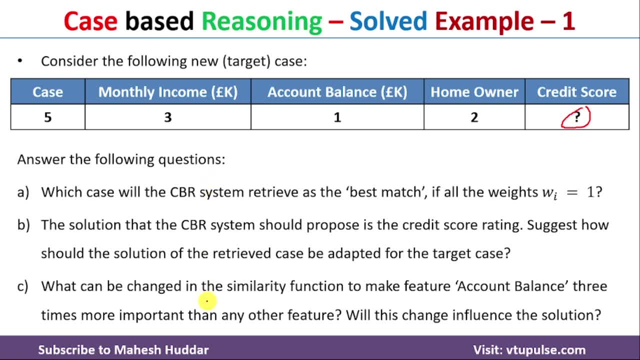 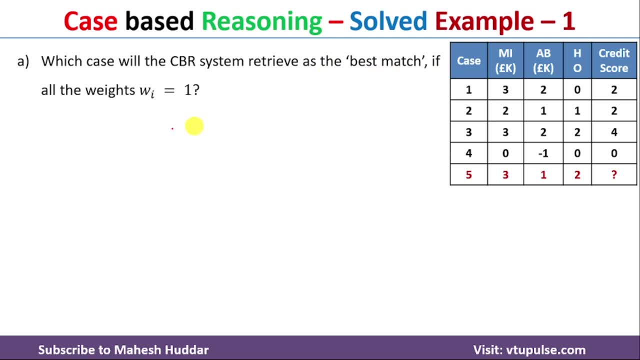 question. We will answer each of these particular questions one by one. The first question is: which case will be the CBR system retrieve as the best match if all the weights are assigned to 1 here? So we will find the distance between the target case and the source And based on that, 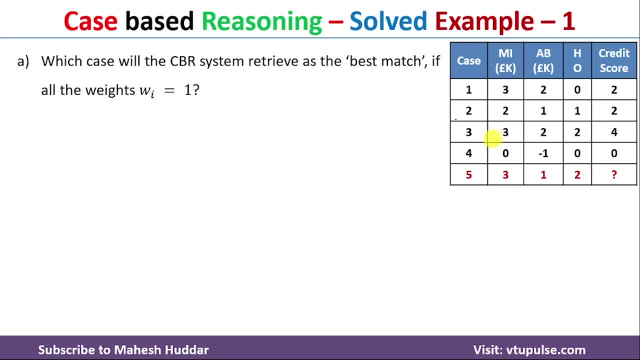 particular distance. we need to select one of these particular case as the best match for this particular new example. So we know how to calculate the distance that is, d of t. s is equal to. summation of i is equal to 1 till m. cardinality of t minus si multiplied. 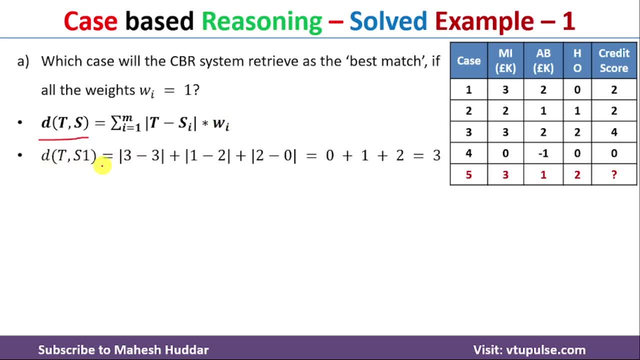 by wi. So we will calculate the d of t s1, that is the distance between t and s, The distance target, and the case 1, which is equivalent to cardinality of t minus si multiplied by wi. so what is t? t in this case, that is 3, si is nothing but the first one, that is 3 here, so 3 minus 3. 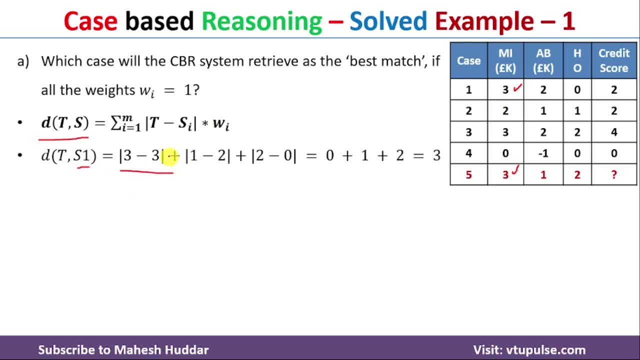 multiplied by wi, wi is equivalent to 1, so that's the reason i have not written here second time. it will be: t is 1 and si will be 2 here. so 1 minus 2, cardinality of 1 minus 2- multiplied by wi. again, it is equivalent to 1. here, coming back to the next one, that is, 2 is the. 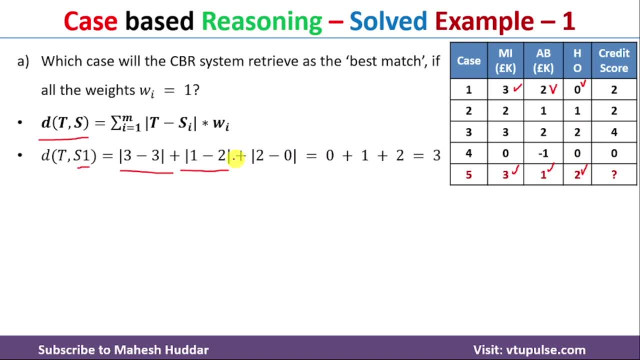 target 0 is the source here. so 2 minus 0- that is what i have written here- multiplied by wi again, which is equivalent to 1. so that's the reason i have not written here, and once you solve it you will get. d of t comma s1 is equivalent to 3 here. similarly, we need to calculate a d of t comma s2. 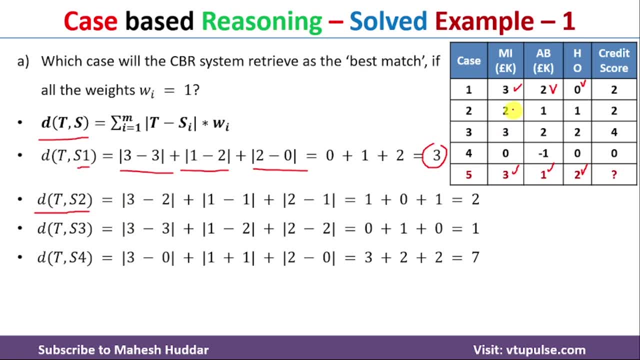 again. t is same here, that is 3, s2 in this case is equivalent to 2, so 3 minus 2, that is what i have written here. you plus 1 minus 1 over here. that is what i have written here, and the last one is 2: 2 minus 1. 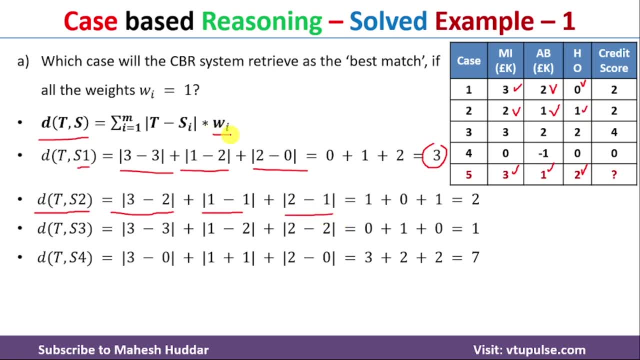 that is what i have written here. everywhere, multiplication factor is wi, which is equivalent to 1. so that's the reason i have not written. so once you solve it, you will get the answer as 2 here. similarly, d of t comma s3. t is common, s3 will be in this case. in the first time it will be 3. 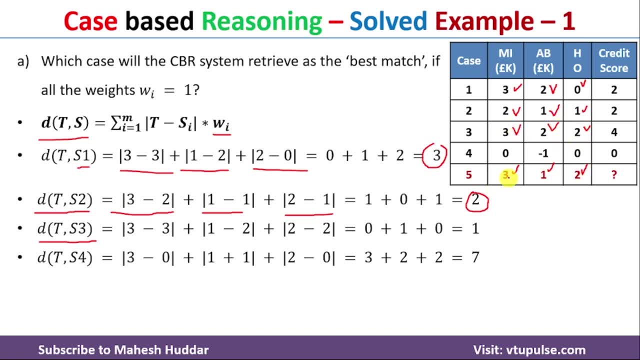 second time it will be 2, and the third time it will be 2 here. so that is nothing but cardinality of 3 minus 3 plus cardinality of 1 minus 2 plus cardinality of 2 minus 2 here. so that is what i have written here, and once you 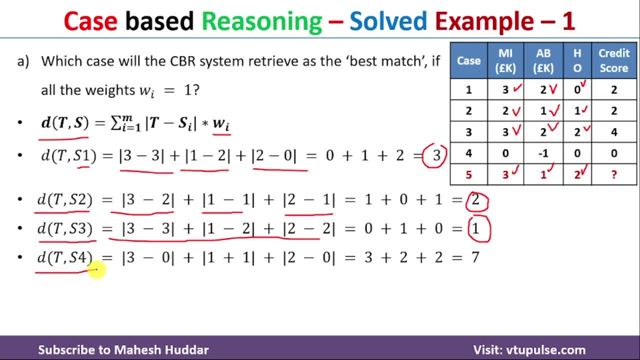 solve it, you will get 1 as the answer. coming back to the last one, that is, d of t comma s4, again t will remain same. s4 in this case is 0 in the first case minus 1 in the second case, 0 in the third. 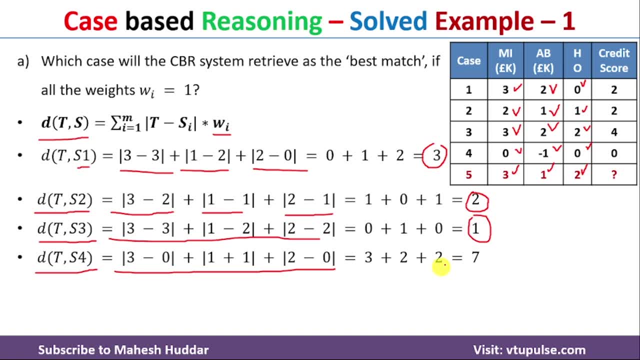 case. so once you put all those party thing in the equation, you will get 7 as the answer in this case. now, if you look at this particular- the distances- the third case is having the smaller value. you can say that the third case is more similar to or best match for the new example in this case. 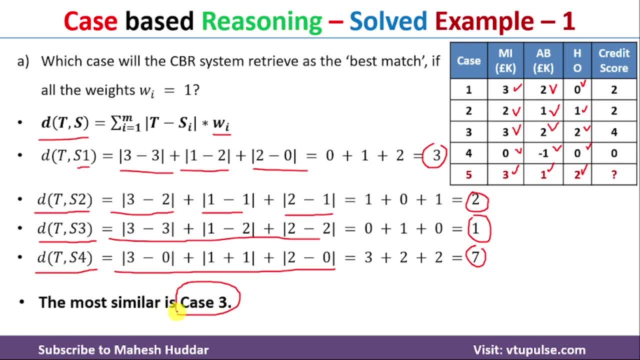 so you can say that the third case is the best case in this case and the credit score of the third case is equivalent to 4, so that will be assigned to this particular the target case over here. the credit score for the target case is equivalent to 4 in this particular case coming. 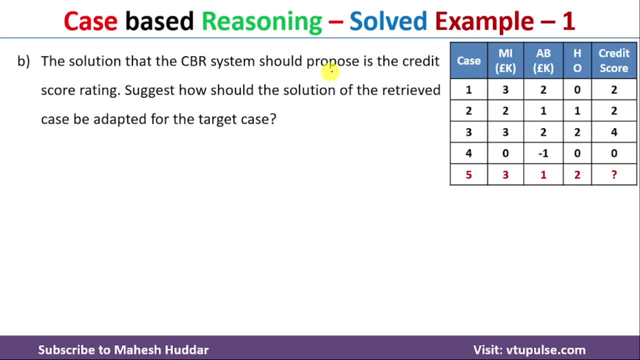 back to the second question. the solution that cbi system should produce is the credit score rating that we have done in the previous slide suggest how should solution of the retrieved case be adapted for the target case, so how we can adapt this particular case, considering this particular. 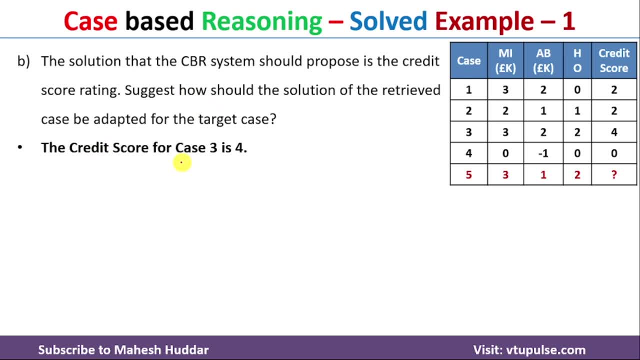 target case. so that is what we need to answer over here. so credit score for the third case is equivalent to what four? that is what we have already identified in the previous case. the only difference between this target case and the third case is- we can see here- the monthly income is 3. 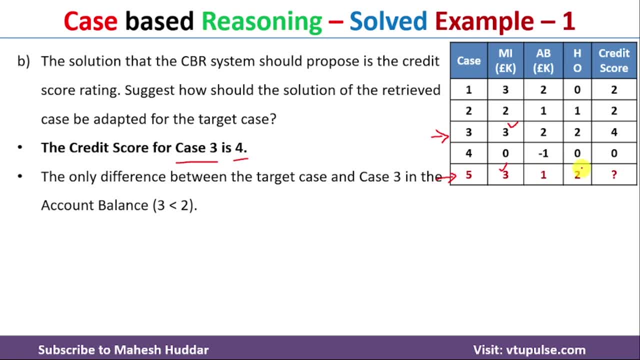 here monthly income is three years, there is no problem. the homeowner is equivalent to 2 here. the homeowner is equivalent to 2 here, but there is a change in this particular account balance. so account balance for third case is equivalent to 2. account balance for this target case is equivalent to 1 here, so that is the only difference. 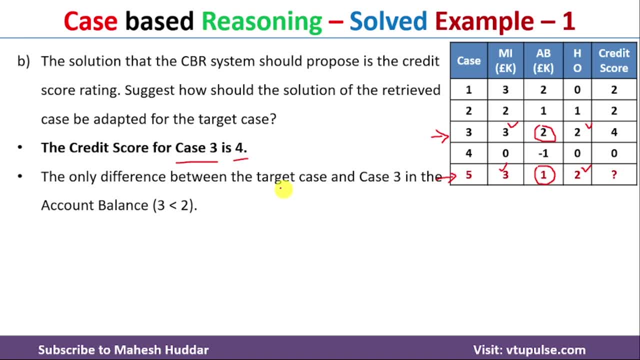 between the third case and the target over here. so what we need to do here is we need to look at other examples with respect to account balance and that credit score and we need to adjust this particular credit score over here. now, if you look at this particular target case- account balance- 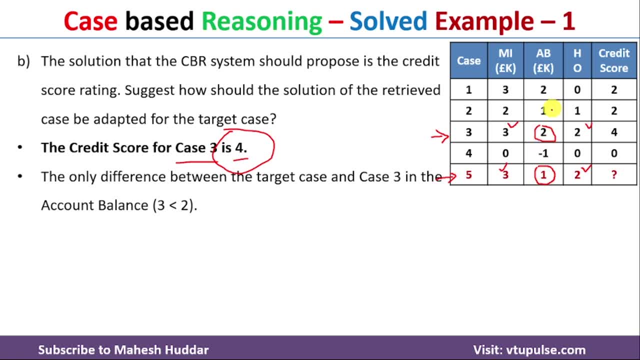 and the account balance of this particular, the source cases. as and when the value of this particular account balance decreases, the credit score is getting decreased. so what is that we need to do? over here is, again, the target case account balance is less compared to the third case, so we need to reduce this particular credit score over here. so, rather than having the credit, 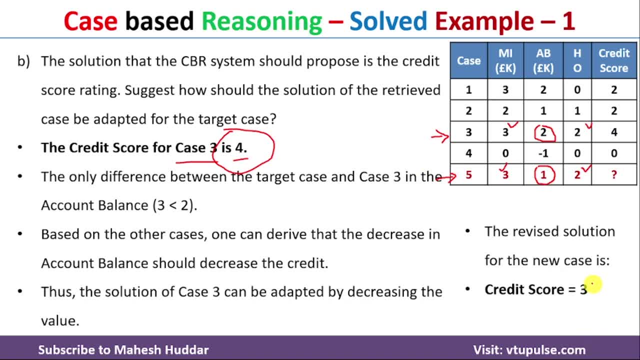 score as 4, it is better to have the credit score equivalent to 3 in this particular case. so this is how actually we can adapt the solution considering this particular target case, in this particular case. now we will answer the third question, that is, what can be changed in the 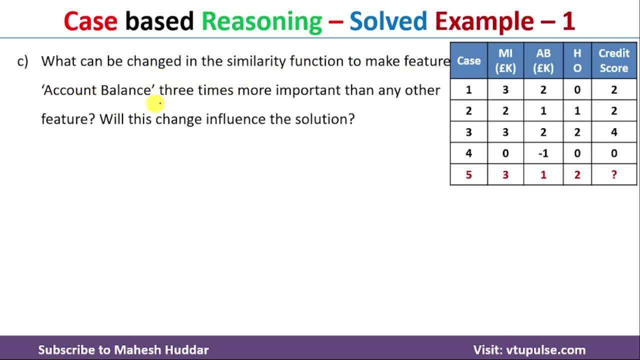 similarity function to make the feature, that is, account balance, three times more important than any other feature. will this change influence the solution? so first, what we need to do here is: in the previous case we have assigned a, wi is equivalent to 1. that is wait for mi, wait for. 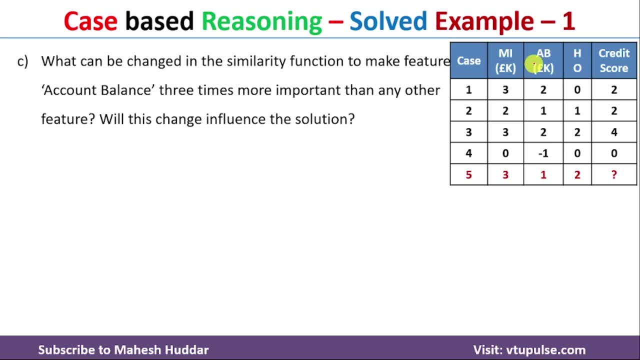 account balance and homeowner. everywhere we have assigned the weight is equivalent to 1. now what they are trying to say is we need to assign the weight for account balance three times the other one. for example, the weight for monthly income is equivalent to 1, weight for homeowner is equivalent. 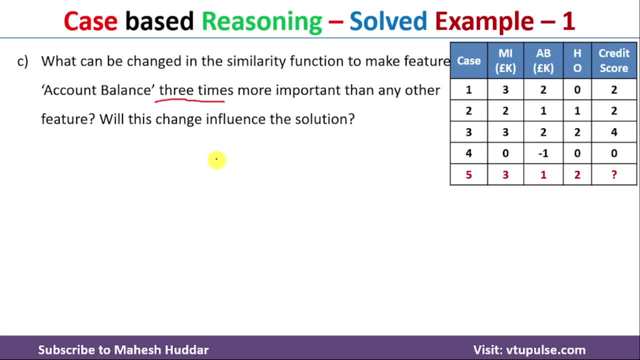 to 1. in that case, the weight for account balance is equivalent to 3 here. so that is how actually we need to change that particular similarity function. and then we need to get the distances. once you get the distance, we need to check whether that modification will influence the 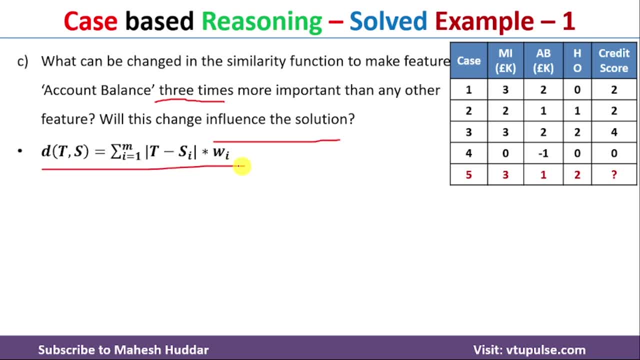 length of that simulation over here. so again we will use this particular similarity function and then we will try to calculate the distance between target and the source here. so target and source, or the case 1, which is equivalent to, again, 3 minus 3 over here multiplied. 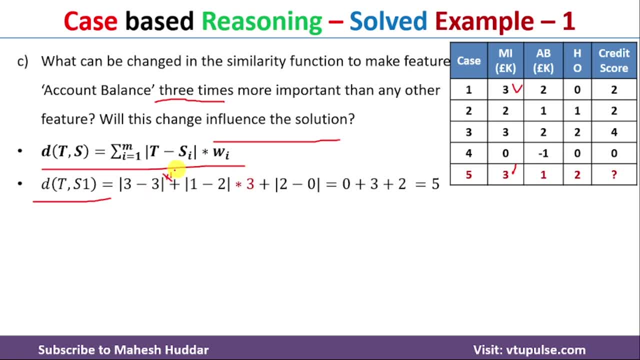 by wi, so w1. in the first case the weight with respect to monthly income is 1, so that they risen multiplication by 1 over here. so that is not required to write 5. coming back to the second one, that is 1 or here and 2 over here. one minus 2 multiplied by wi. what is it 1 here? so that is a multiplication paid over here and 2 over here. 1-2 multiplied by wi. what is it 1 over here is to 3cesso twice, which actually is less than multiply and error 32.. 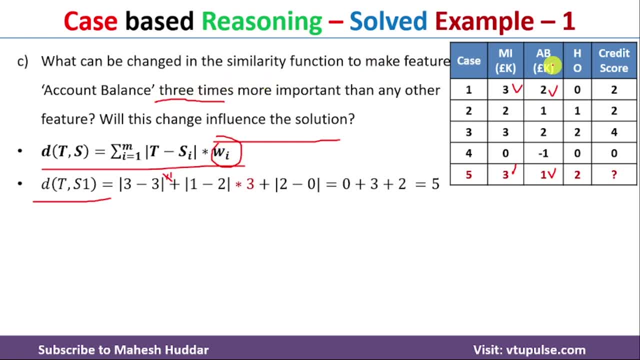 what is that wi? the wi is 3 because the account balance weight is equivalent to 3 here. so that is what i have written with red color here. so cardinality of 1 minus 2 multiplied by 3 here coming back to the last one, that is 2 minus 0, that is cardinality of 2 minus 0 multiplied by wi. 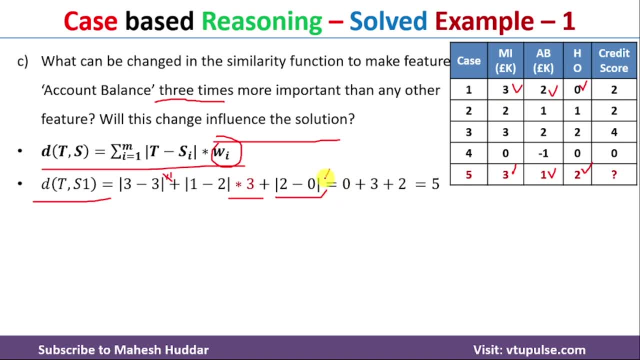 again, the weight with respect to homeowner is equivalent to 1, so that is not required to be written here. so once you solve this party thing, you will get 5 as the answer here. similarly, we need to get the values or the distances for the second case, third case and the fourth case. we got